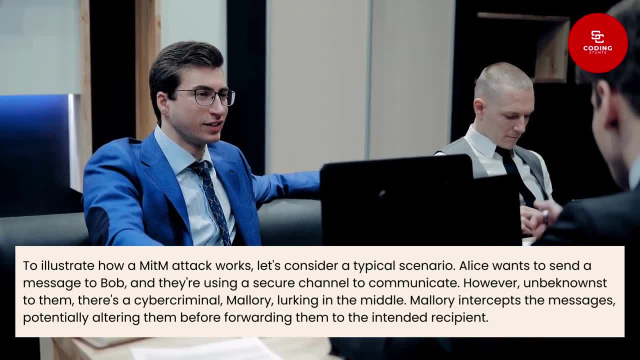 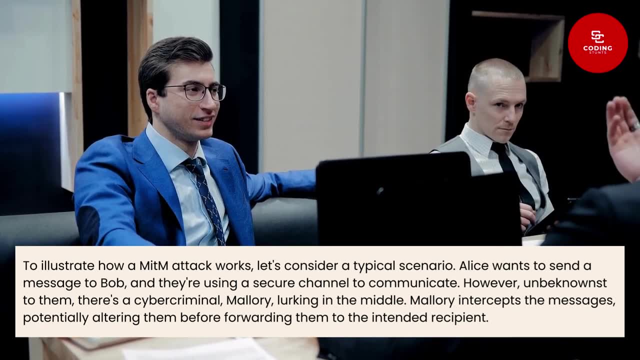 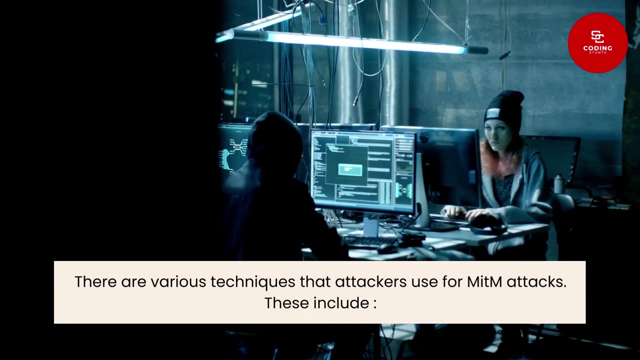 undisgnosed to them. there's a cyber criminal, Mallory, lurking in the middle. Mallory intercepts the messages, potentially altering them, before forwarding them to the intended recipient. Common techniques: There are various techniques that attackers use for MITM attacks. 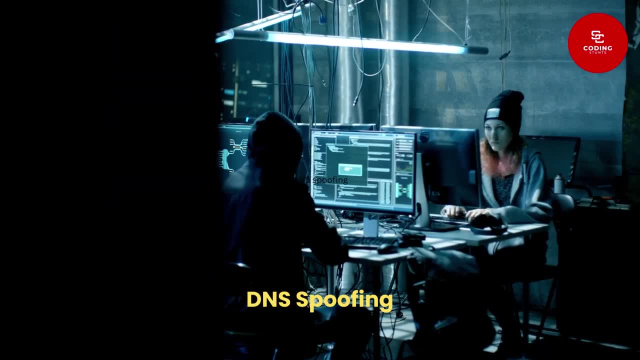 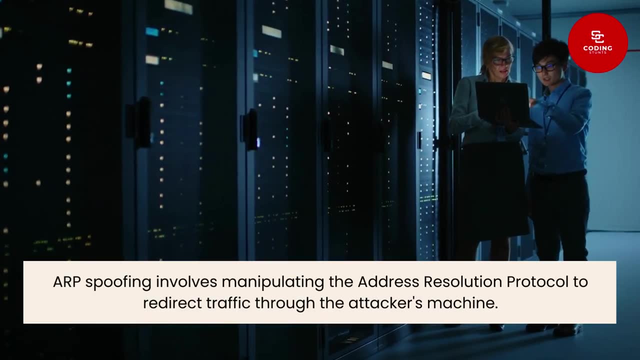 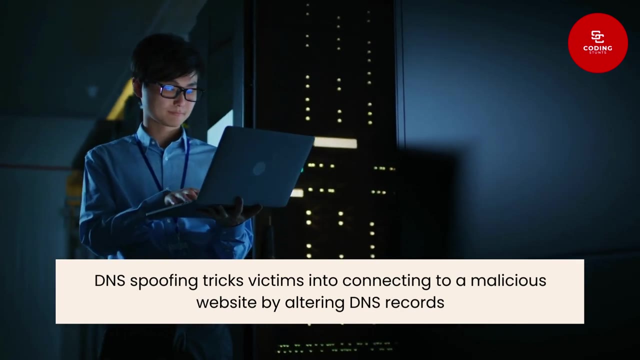 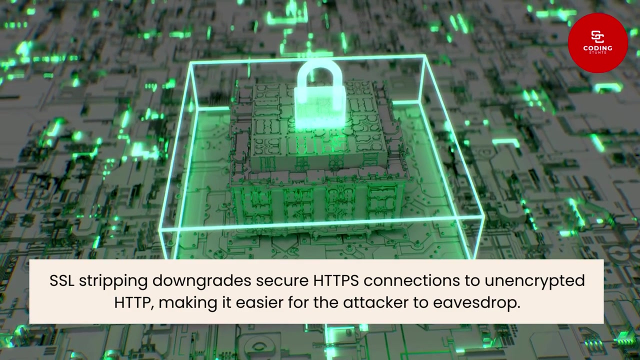 These include ARP spoofing, DNS spoofing and SSL stripping. ARP spoofing involves manipulating the address resolution protocol to redirect traffic through the attacker's machine. DNS spoofing tricks victims into connecting to a malicious website by altering DNS records. SSL stripping downgrades secure HTTPS connections to unencrypted HTTP, making it easier for the attacker to eavesdrop. 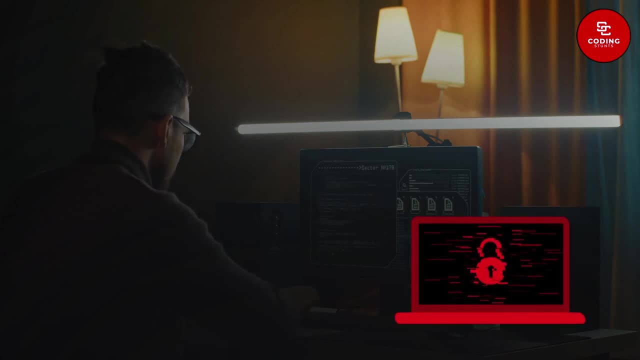 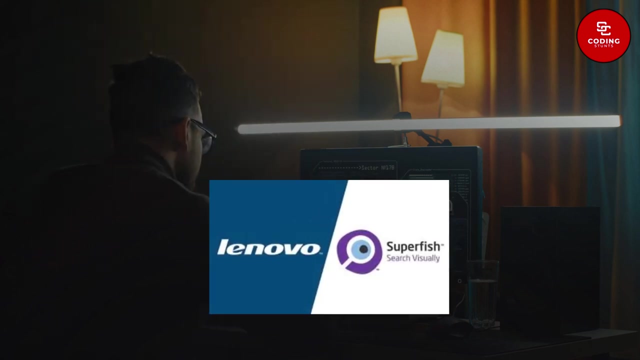 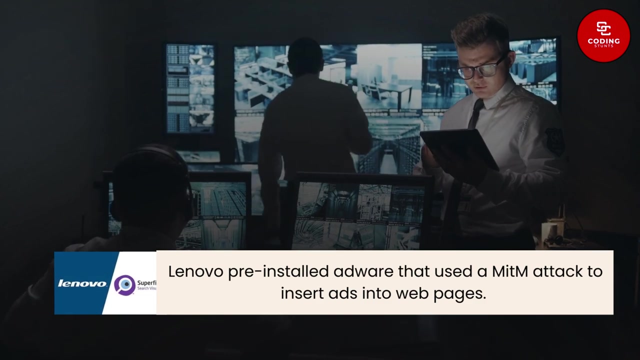 Let's talk about some real-world examples. Now that we understand how MITM attack works, let's look at some real-world examples like Remember the Superfish adware scandal, Lenovo pre-installed adware that used a MITM attack to insert ads into webpages. 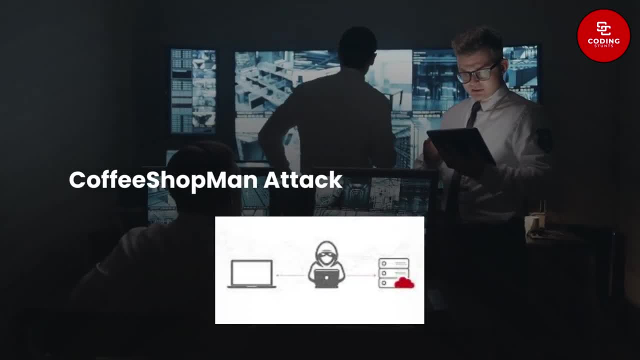 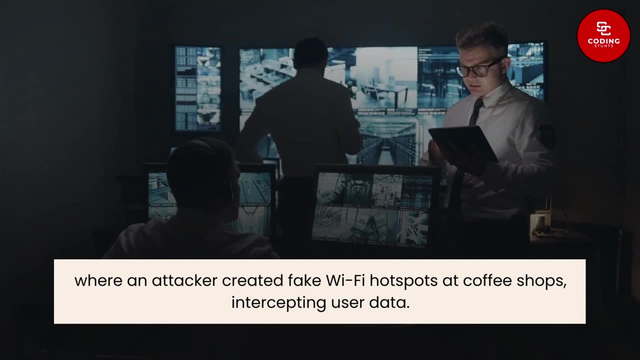 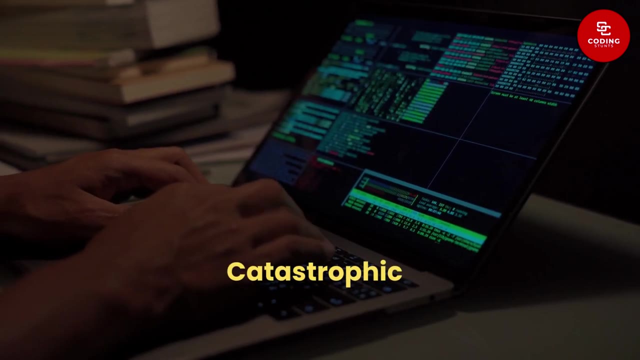 Another example: The Coffee Shop Man attack, where an attacker created fake Wi-Fi hotspots at coffee shops, intercepting users' data. Consequences: The consequences of falling victim to a MITM attack can be catastrophic. Attackers can steal sensitive information like login credentials, financial details or personal data. 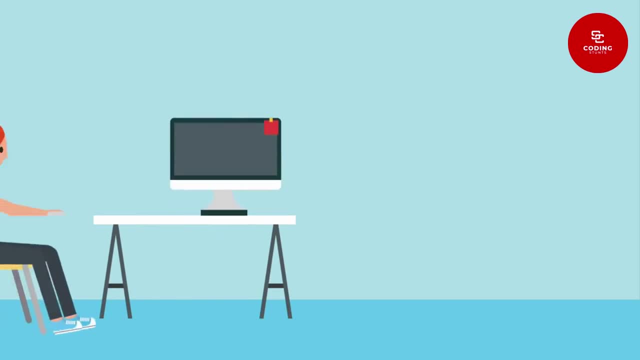 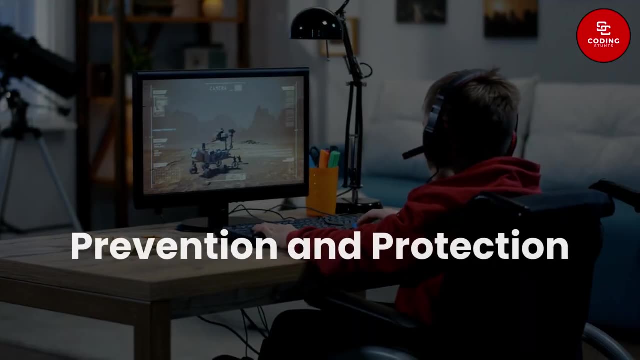 They can also inject malware into your device or manipulate communications to their advantage, Causing reputational damage. Preventions and protections. But fear not, there are ways to protect yourself from MITM attacks. Here are some crucial tips: 1. Use encryption. 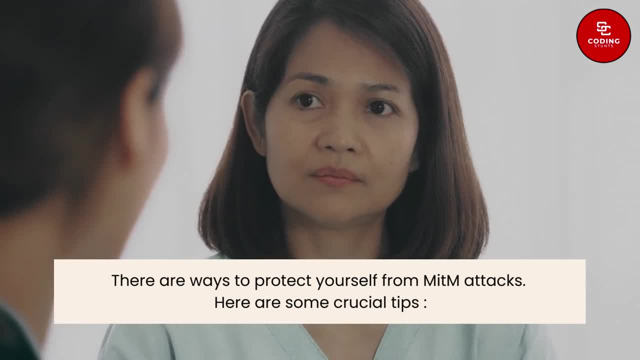 Always OTP for secure encrypted communication channels like HTTPS. 2. Verify certificates: Ensure that websites have valid SSL certificates. 3. Be cautious on public Wi-Fi. Avoid conducting sensitive transactions. 4. Be cautious on the use of public Wi-Fi. 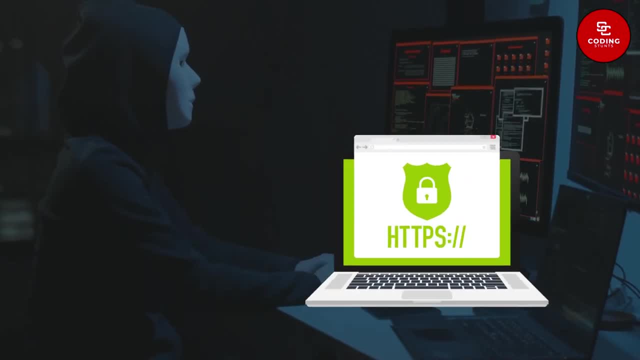 5. Be cautious on the use of public Wi-Fi. 6. Be cautious on the use of public Wi-Fi. 7. Be cautious on the use of public Wi-Fi. 8. Be cautious on the use of public Wi-Fi. 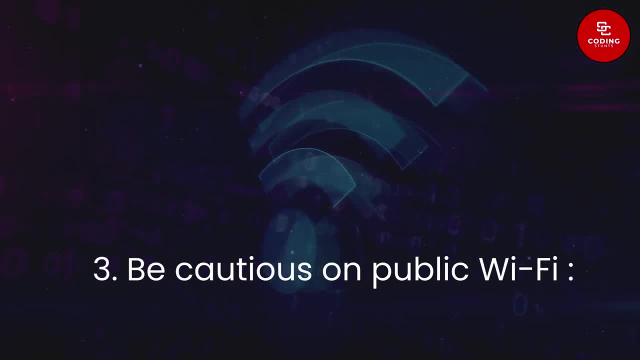 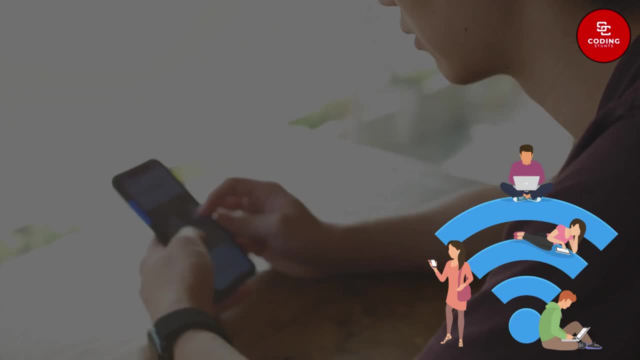 9. Be cautious on the use of public Wi-Fi. 10. Be cautious on the use of public Wi-Fi. 11. Be cautious on public Wi-Fi. Avoid conducting sensitive transactions or unsecured public networks. 4. Install security software.